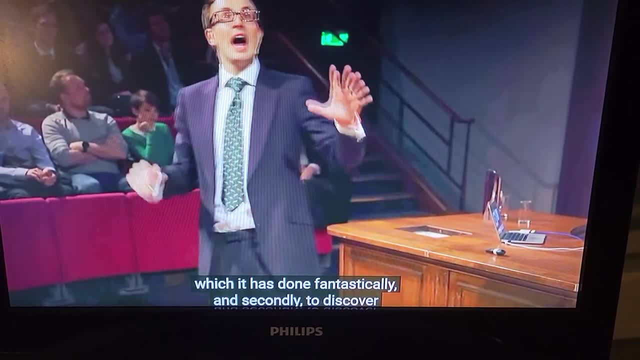 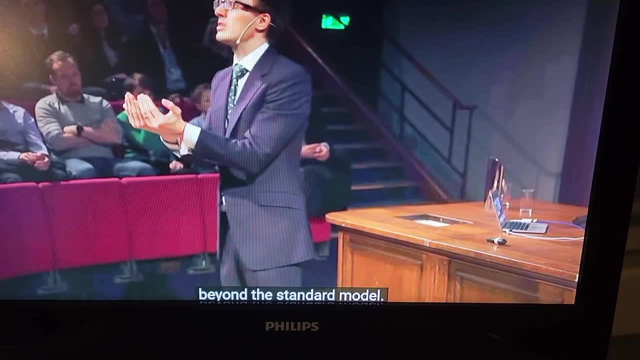 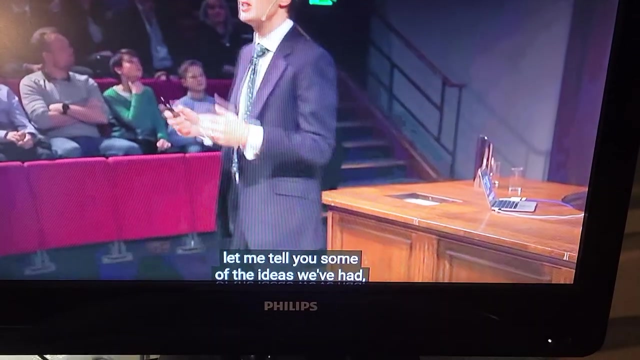 understand the Higgs better- which it's done fantastically- and secondly, to discover new physics that lies beyond the Higgs, new physics beyond the standard model. So, before I tell you what it's seen, let me tell you some of the ideas we had, some of our expectations and hopes. 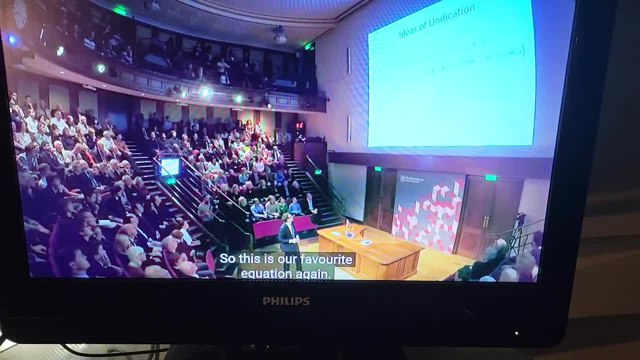 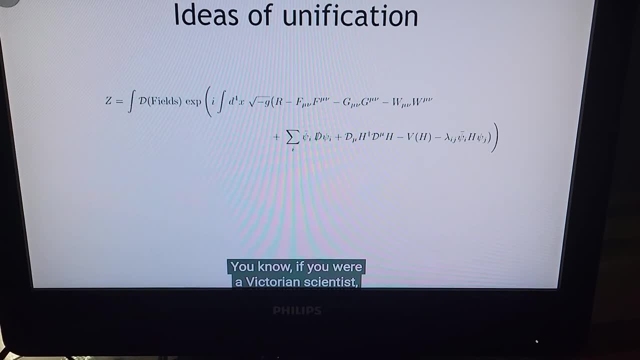 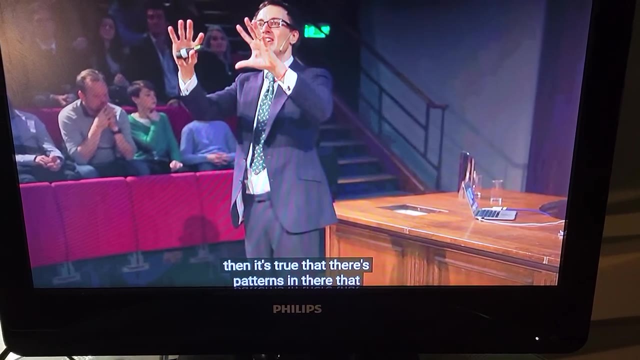 for what would happen moving forward. So this is our favorite equation again. The idea has always been the following: You know, if you're a Victorian scientist and you go back and you look at the periodic table of elements, then it's true that there's patterns in there that give a hint of the structure that lies underneath. 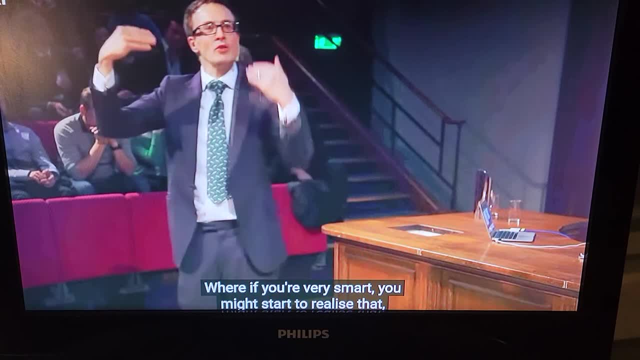 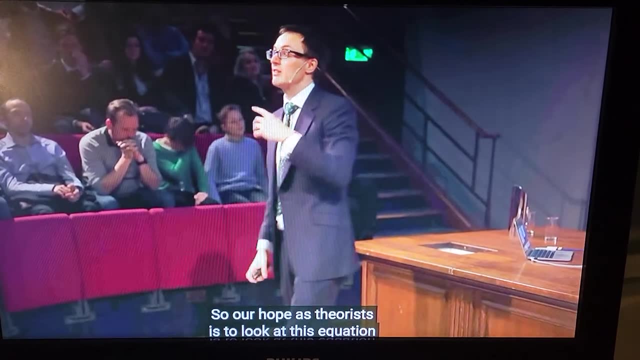 There's numbers that repeat themselves where, if you're very smart, you might start to realize that you know. yes, there is something deeper than just these elements. So our hope as theorists is to look at this equation and see if maybe we can just find patterns in this equation. 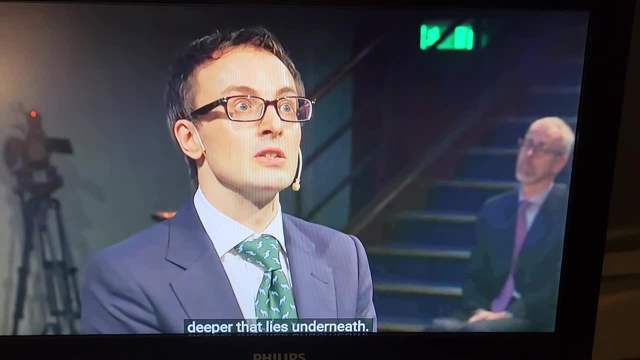 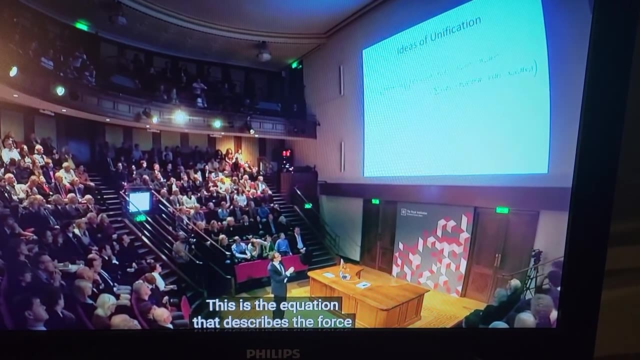 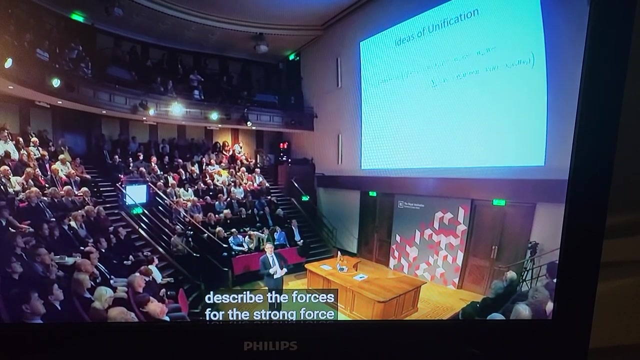 that suggest there might be something deeper that lies underneath, And they're there. So let me give you an example. This is the equation that describes the force of electricity and magnetism, And it's almost the same as the equations which describe the forces for. 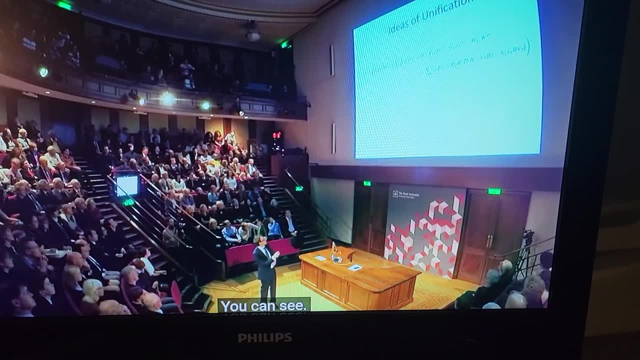 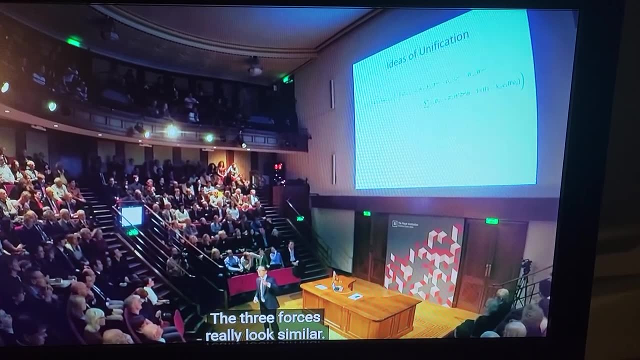 the strong force and the weak nuclear force. In fact you can see I've just changed letters. It's a little more complicated than that, but it's not much more complicated than that. The three forces really look similar. So you might wonder: well, maybe there's not three forces in the unit. 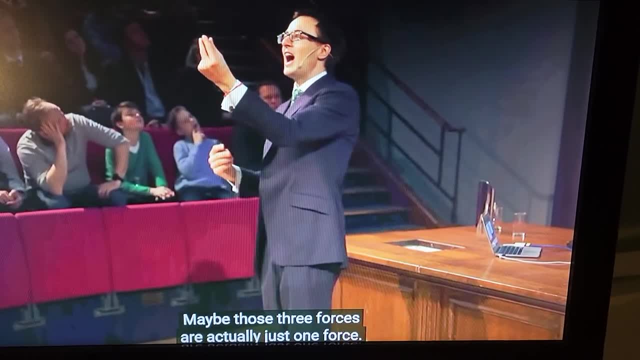 Maybe there's so soțes that run into the interest of the universe, But there's only one force in my image. Maybe those three forces are actually just one force, And when we think there's three forces it's because we're looking at that one force just from. 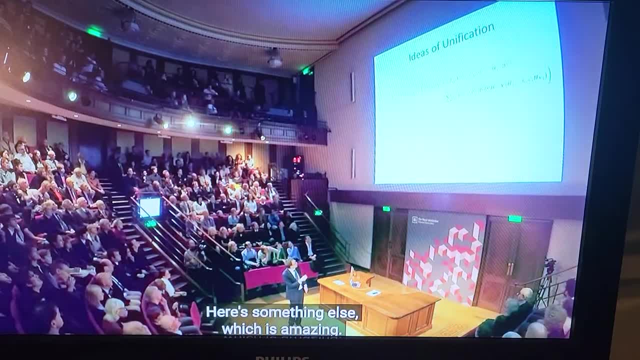 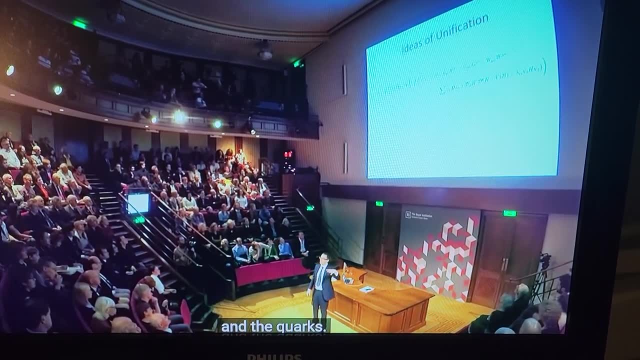 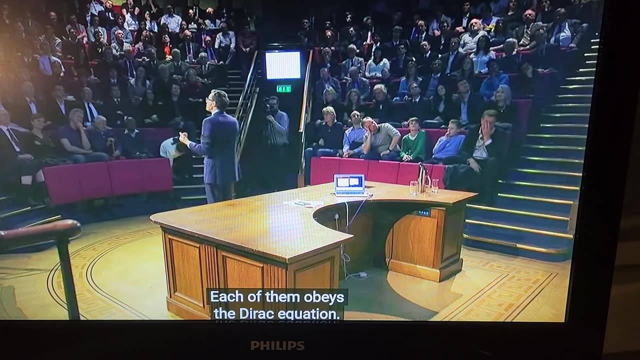 slightly different perspectives. Maybe Here's something else which is amazing. These are the equations for the 12 matter fields in the universe: the neutrinos, the electrons and the quarks. Each of them obeys exactly the same equation. Each of them obeys the Dirac equation. 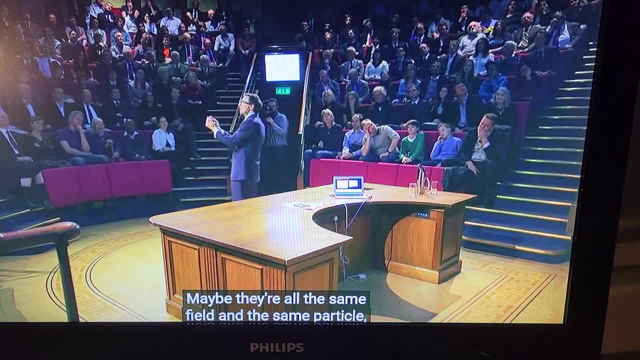 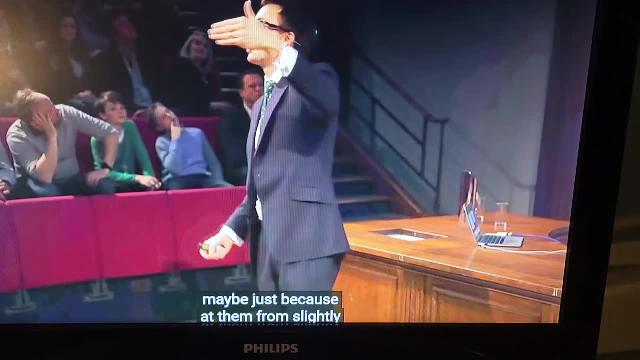 So again you might wonder that well, maybe there aren't 12 matter fields, but well, they do 12 different fields. maybe they're all the same field and the same particle and the fact they look different is, again, maybe just because we're looking at them from slightly. 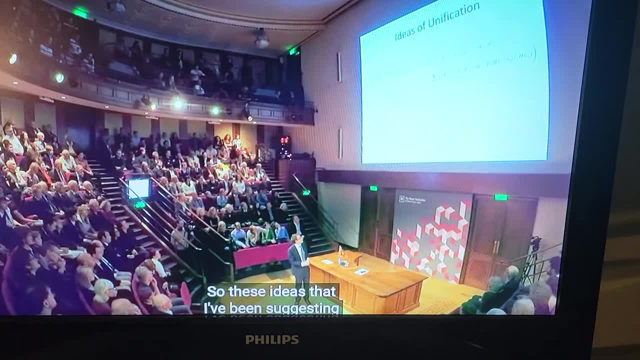 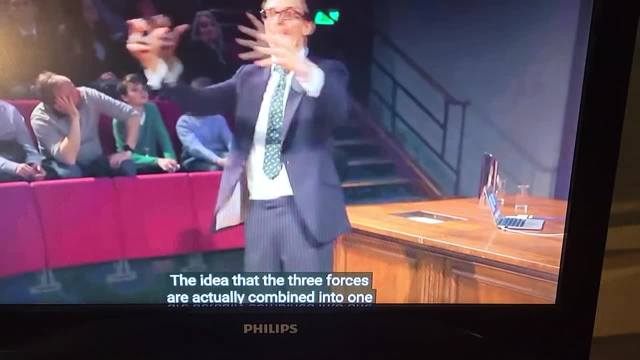 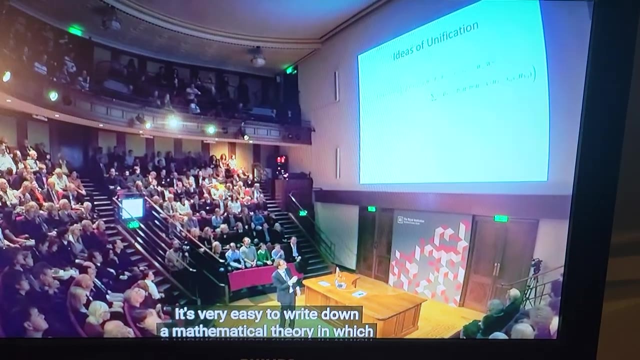 different perspectives, Maybe. So these ideas that I've been suggesting go by the name of unification. The idea that the three forces are actually combined into one is what's called grand unification, And it's very easy. it's very easy to write down a mathematical theory. 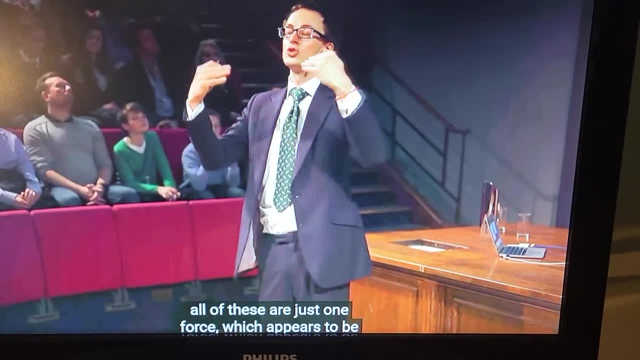 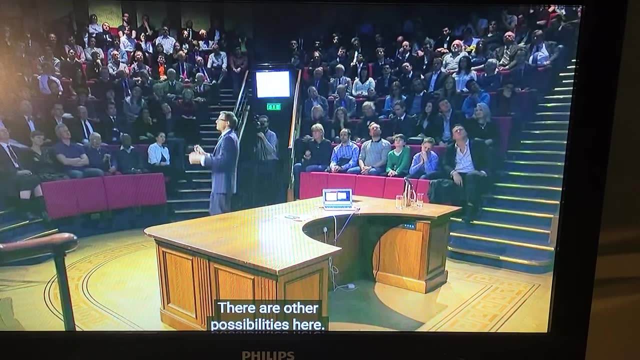 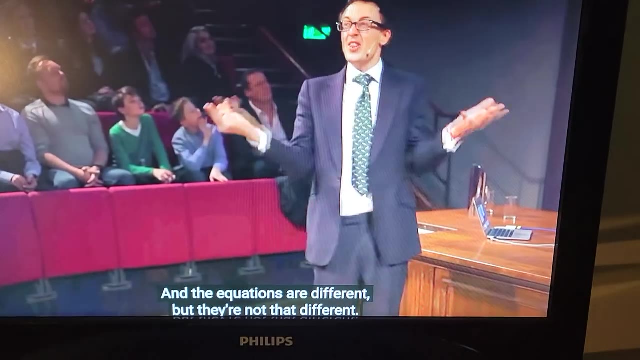 in which all of these are just one force, which appears to be three from our perspective. There are other possibilities here You might say: well, this is the matter and these are the forces, and the equations are different, but they're not that different because, ultimately, 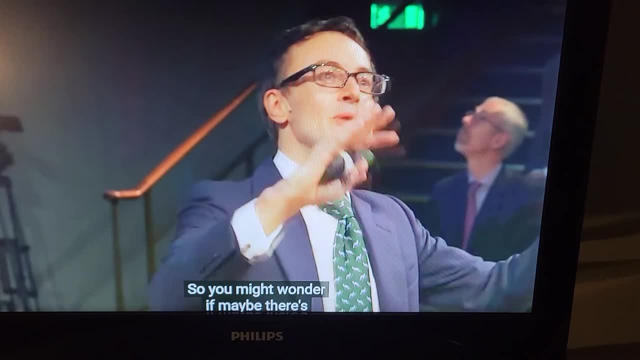 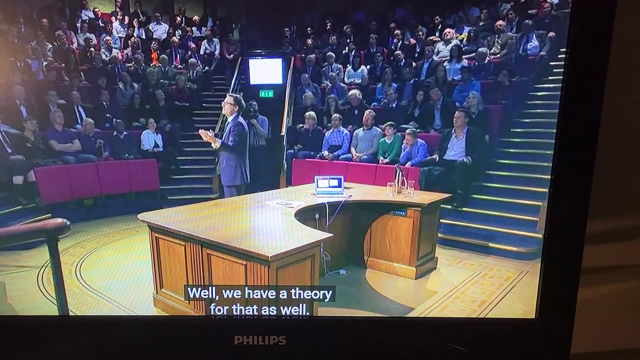 they're both just fields. So you might wonder if maybe there's some way in which the matter and the forces are related to each other. Well, we have a theory. We have a theory for that as well. It's a theory that's called supersymmetry, And it's a beautiful 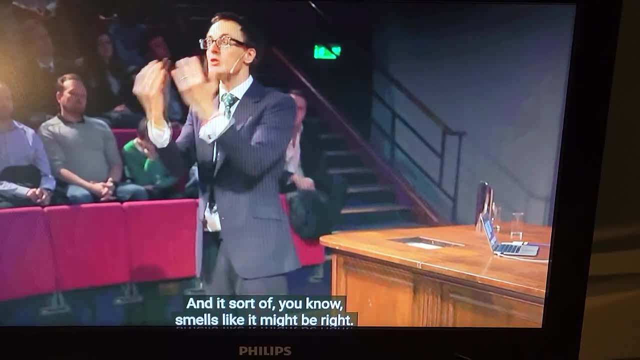 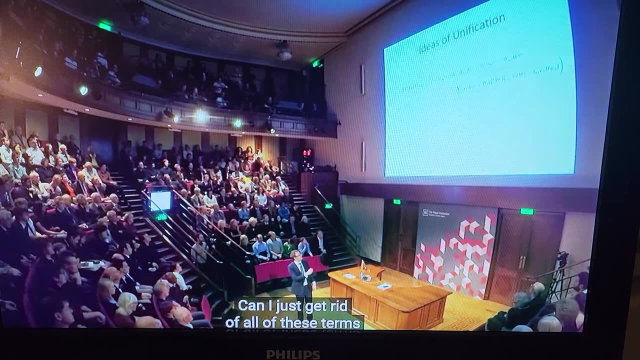 theory. It's very deep conceptually and it sort of smells like it might be right. Finally, you might be really, really bold. You might say: well, can I just combine the lot? Can I just get rid of all of these terms and just write down one single term from which everything? 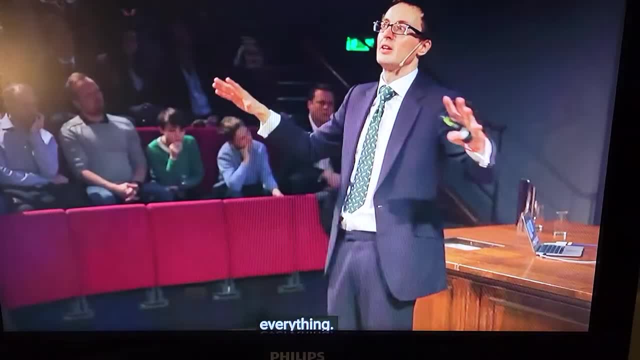 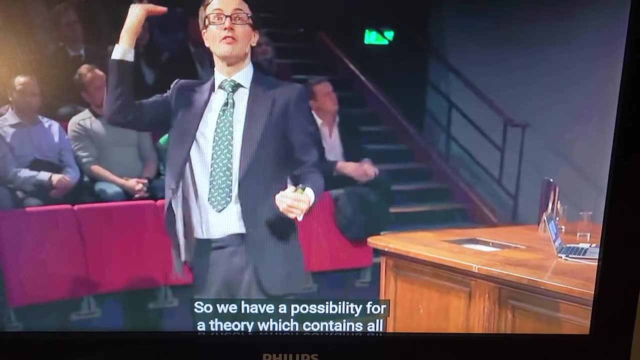 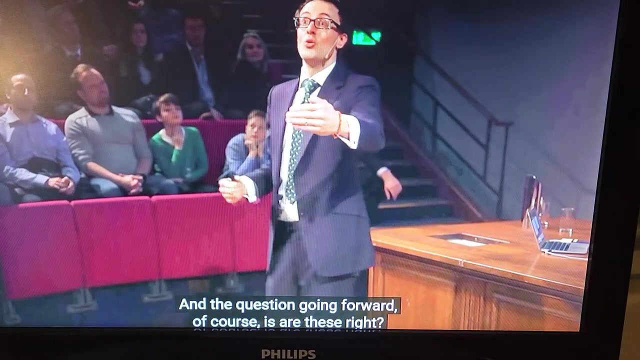 else emerges: Gravity, the forces, the particles, the Higgs, everything. Well, I've got something for you if you want that as well. It's called string theory. So we have a possibility for a theory, And then of course, of course, we've got austereate back Right, So string theory contains a matrix. 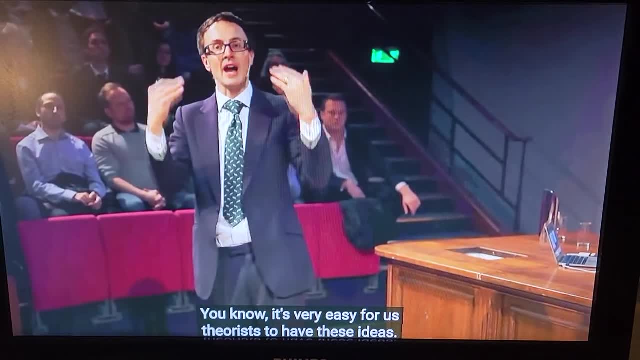 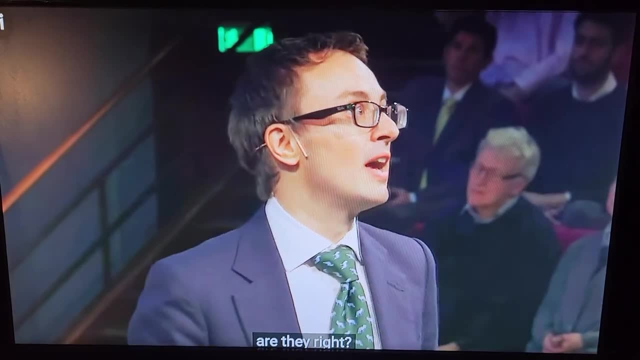 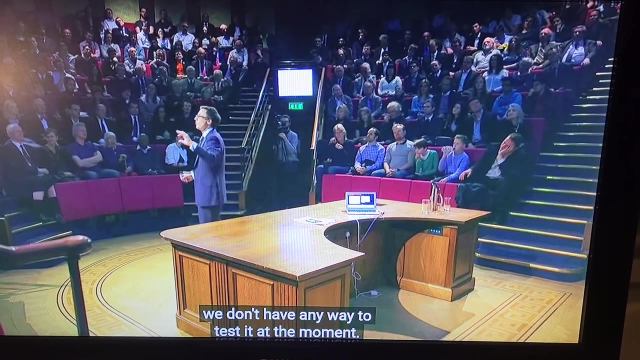 called perceptron, a gradu eigen automata, which contains all of this in one simple concept. And the question going forward, of course, is: are these right? It's very easy for us theorists to have these ideas, And I should say these ideas are what's driven theoretical. 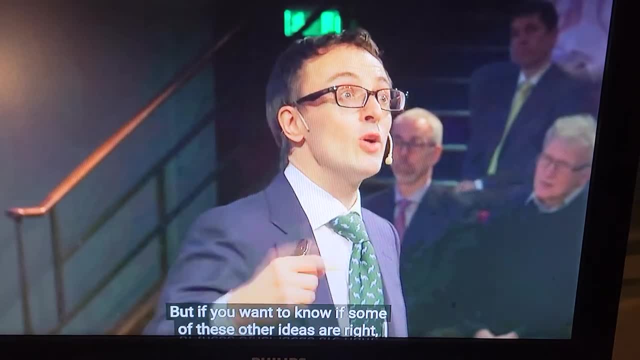 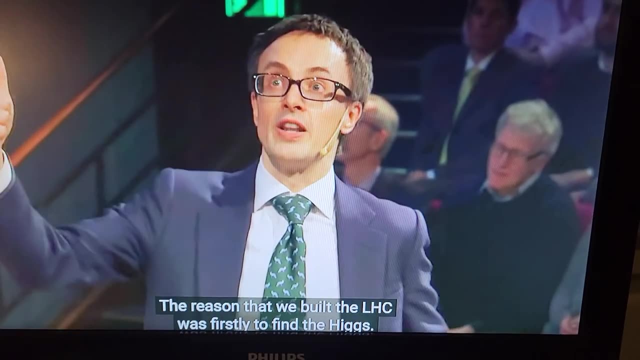 physics for 30 years, but we want to know, are they right? And we've got a way of telling This: right are right, then that's what the lhc should be doing. the reason that we built the lhc was firstly to. 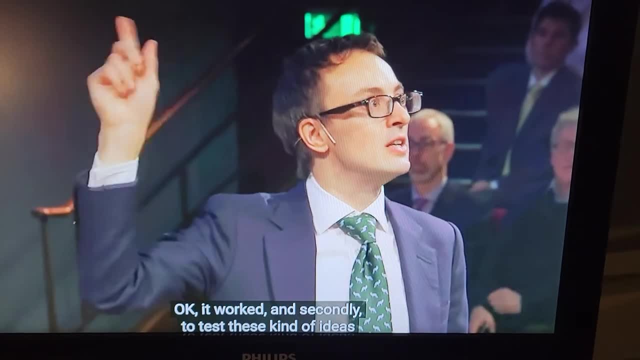 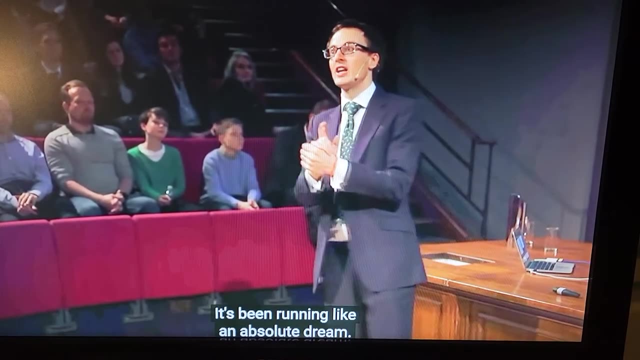 find the higgs okay, it worked. and secondly, to test these kind of ideas that we've been having to see what lies beyond. so the lhc has been running. it's been running for two years. it's been running like an absolute dream. it's just, it's a perfect machine. uh, two years, uh, this is. 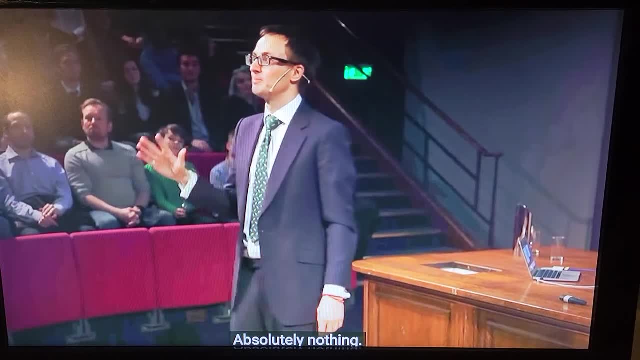 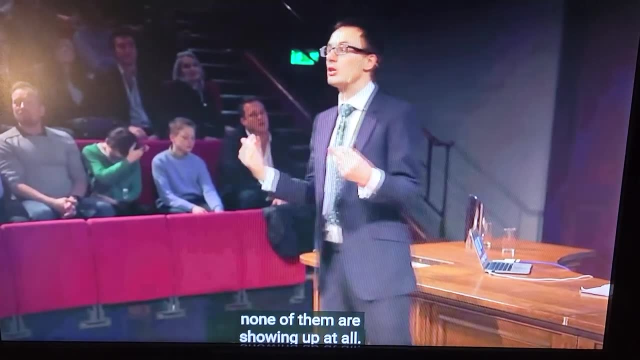 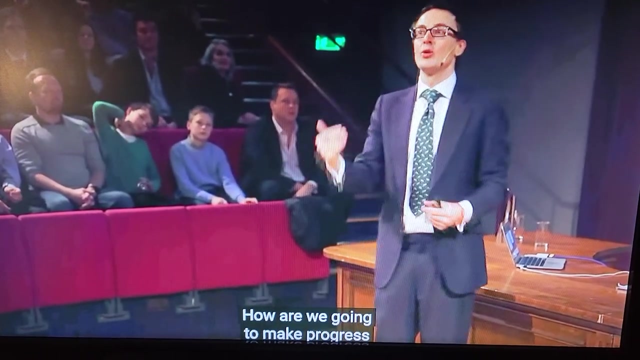 what it's seen? absolutely nothing. okay, all of these fantastic, beautiful ideas that we've had, none of them are showing up at all, and the question going forward is: you know what are we going to do about it? uh, you know how are we going to make progress in understanding the next? 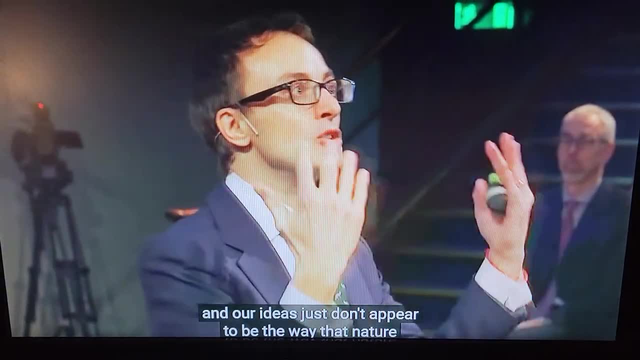 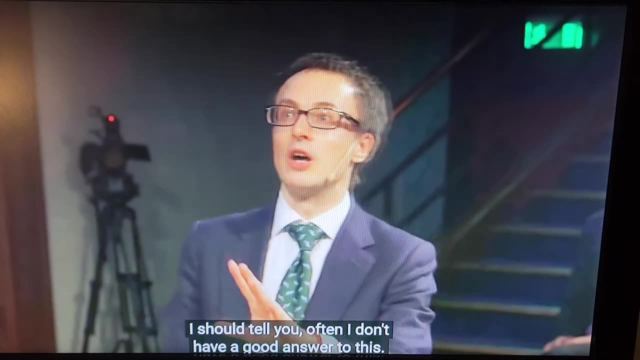 layer of physics, when the lhc isn't seeing anything and our ideas just just don't appear to be, uh, the way that nature works. okay, i should tell you, often i don't have a good answer to this. um, it's uh, i say my impression is that most of my community is a little bit shell-shocked by 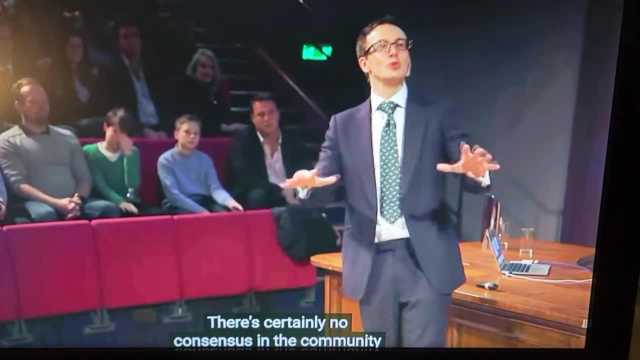 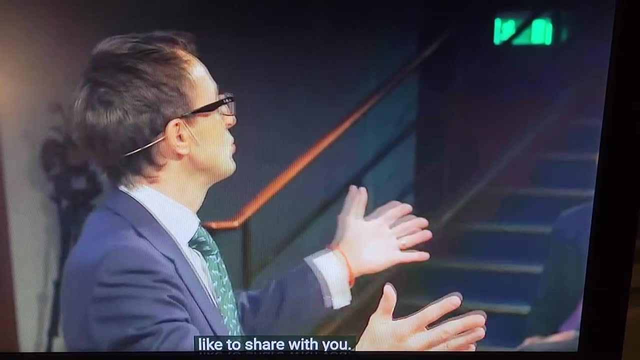 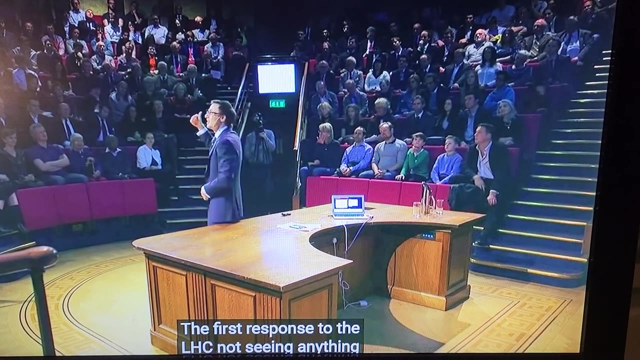 by what happened. um, there's certainly no consensus in the community to move forward, but i think there's three responses that that sort of various people have had that i'd like to share with you. i think all three of these responses are reasonable up to a point. um, the first response to the lhc not seeing anything. 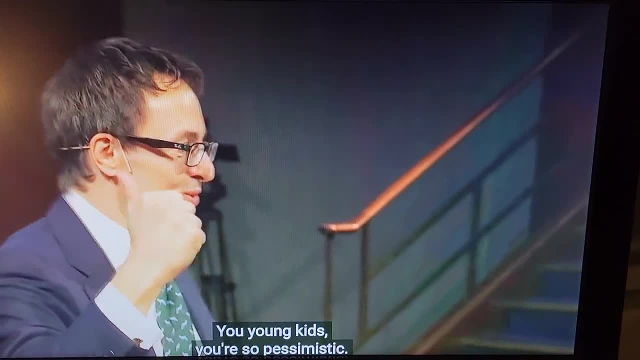 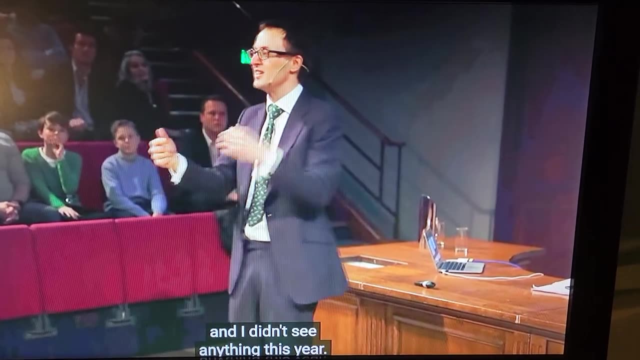 is the following: it's: um well, you know you, you young kids, you're so pessimistic. it's all doom and gloom with you. you just you need a little bit more patience. you know it didn't see anything last year, it didn't see anything this year, but but next year it's going to be a little bit more. 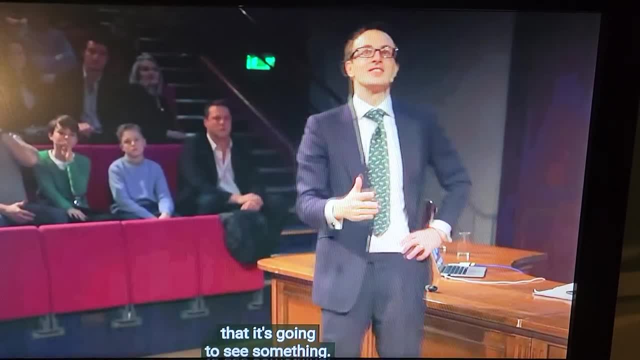 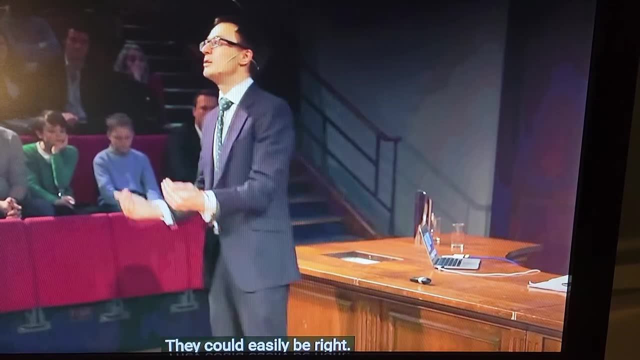 it's going to see something and if not next year, it's the year after that that it's going to see something. it's it's usually my, my very illustrious senior colleagues that that have this, this response, and you know what? they could easily be right. it could easily be that next year, the lhc. 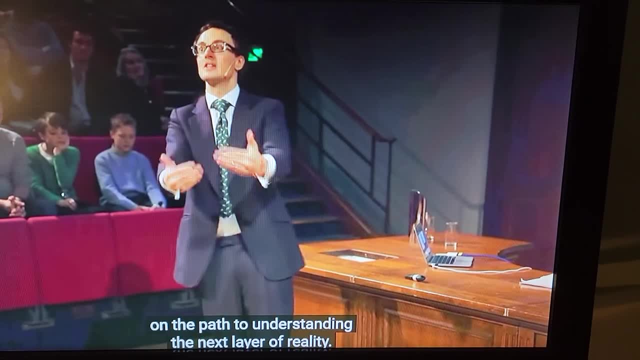 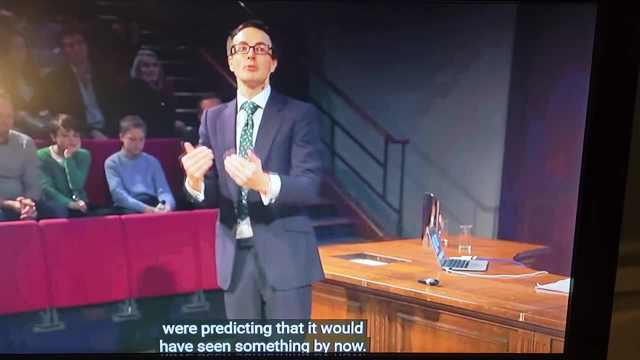 discovers something astonishing, and it sets us on the path to understanding the next layer of layer of reality, um, but it's also true that these same people were predicting that it would have seen something by now, and it's also true that, um, this can't keep going for much longer, and 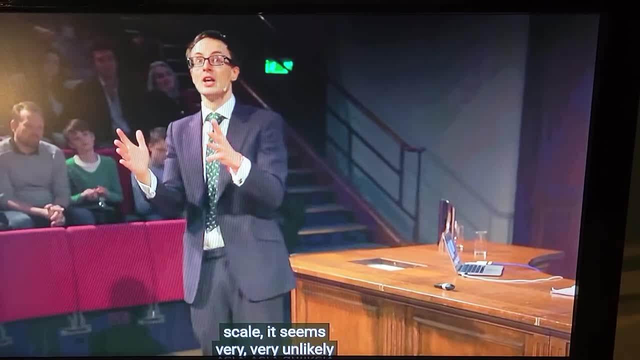 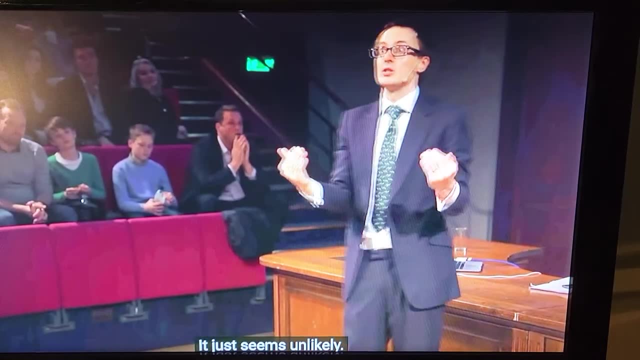 longer. if the lhc doesn't see something within, say, a two-year time scale, it seems very, very unlikely that it's going to see something moving forward. it's possible, it just seems unlikely. so, uh, you know, we'll know. i i hope with all my heart that the lhc discovers something next year or the year. 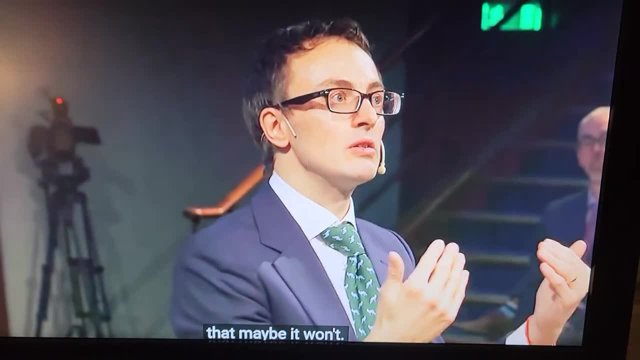 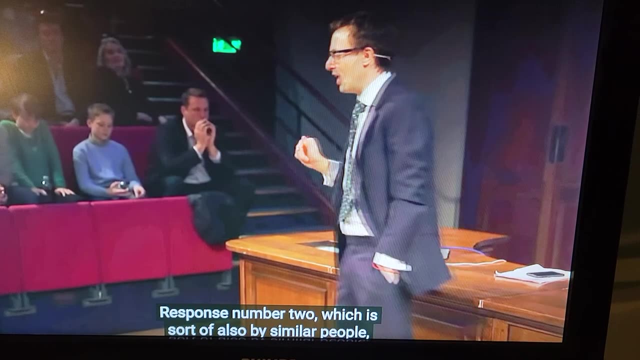 after: um, but i think we have to prepare for, for the worst, that that maybe it won't okay. response number two: uh, response number two, which is sort of also by, by similar people: um well, all our theories are so beautiful, they absolutely have to be correct, and what we really need is a bigger machine. 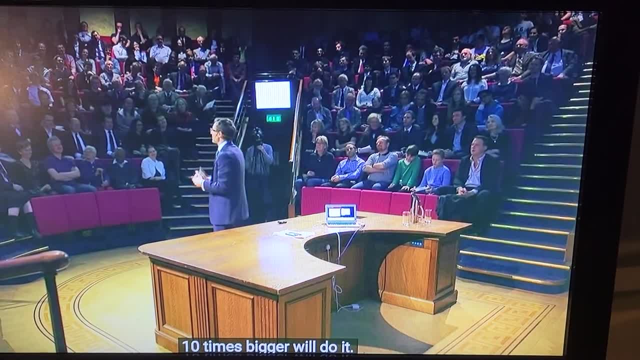 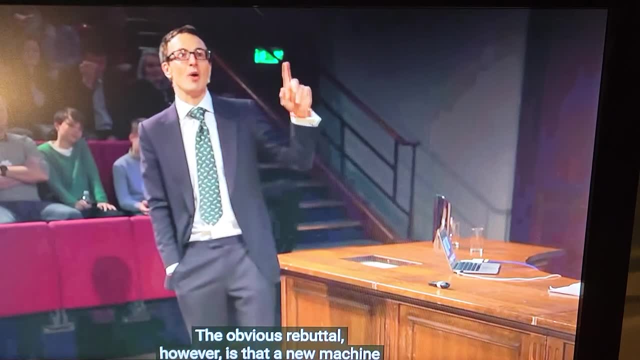 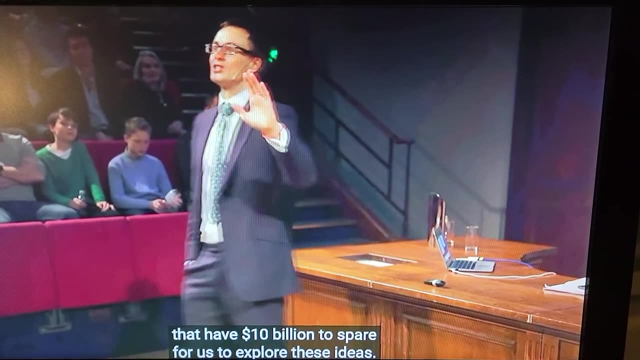 uh, ten times bigger, we'll, we'll do it okay again. they, they, they might be right. i don't have a good argument against it, uh. the obvious rebuttal, however, is that a new machine costs 10 billion dollars, and there's not too many governments in the world that have 10 billion dollars to spare for us to. 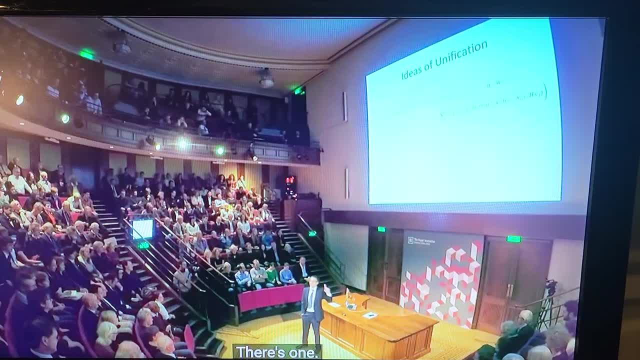 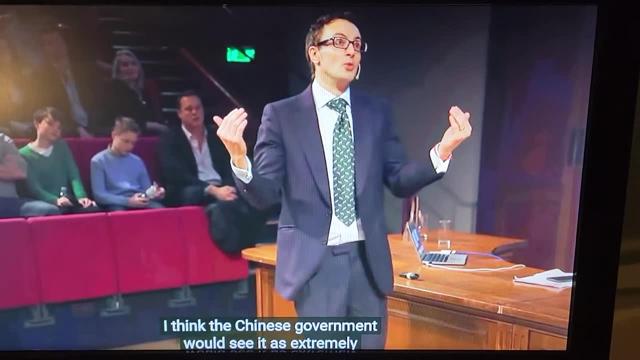 us to explore these ideas. there's one, uh, the one is china, and so if this machine is going to be built at all, it's going to be built by the chinese government and it's going to be built by the chinese government. i think the chinese government would would see it as extremely attractive if the 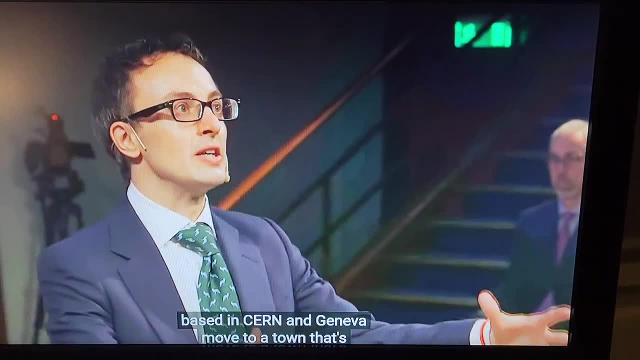 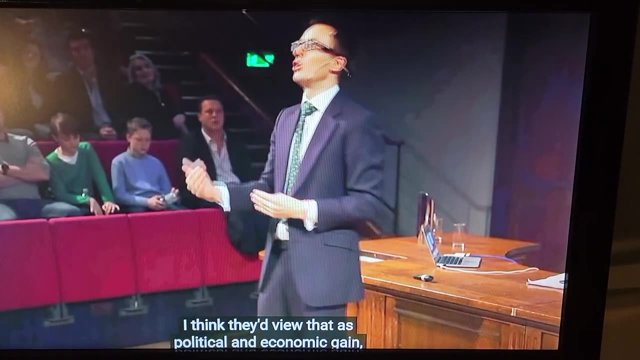 whole community of uh particle physicists and engineers that are currently based in cern and geneva uh move to a town that's slightly north of beijing, i think. i think they'd uh view that as a political and economic gain and there's, you know, a real chance they may decide to build this machine. 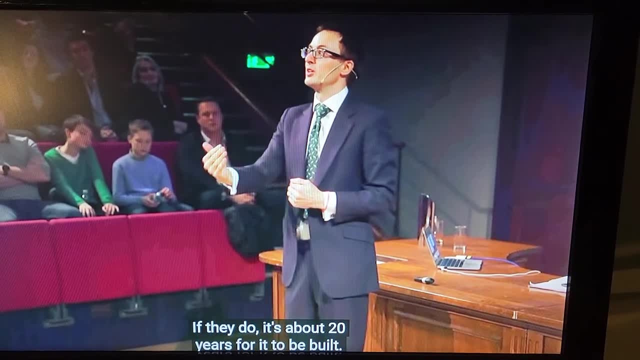 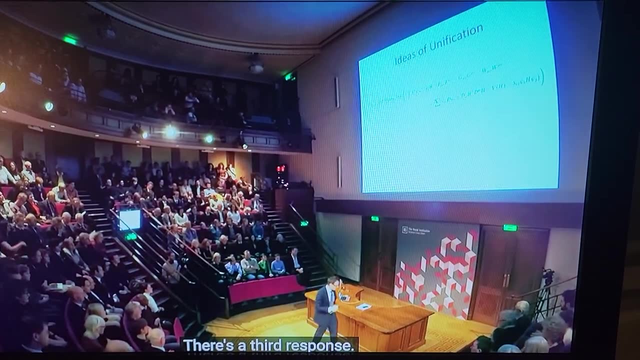 if they do, it's about 20 years, uh, for it to be built. so, uh, we're waiting slightly longer. uh, there's a third response. um, i should say the third response is is kind of the camp i'm in. um, i should mention up front it's. 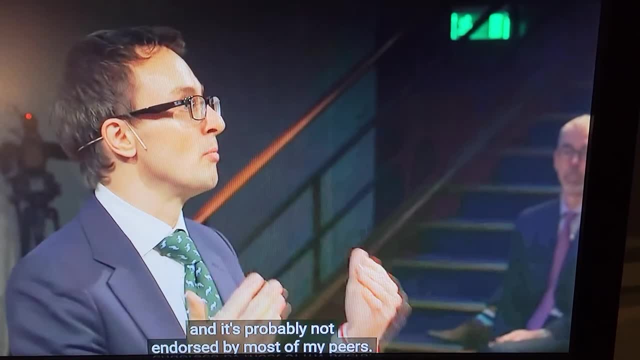 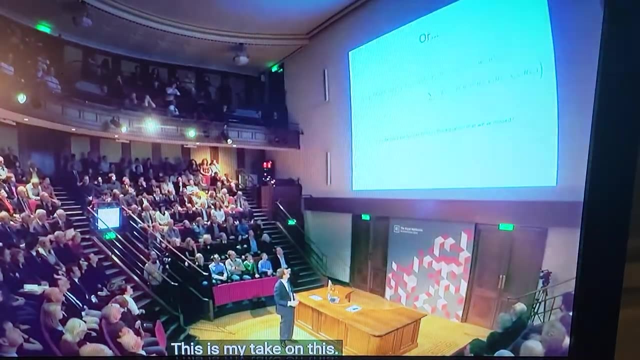 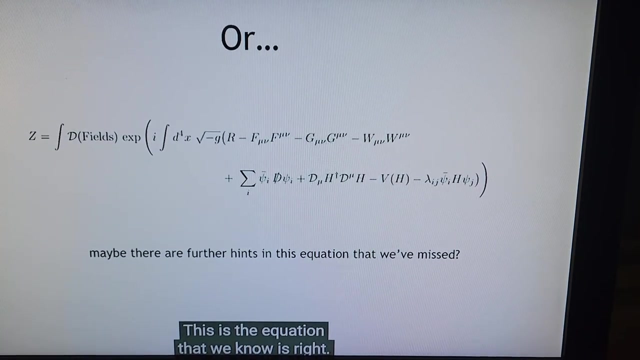 speculative and it's probably not endorsed by most of most of my peers. so this is really just my personal opinion at this point. um, this is my take on on this. um, this is, you know, uh, this is the equation that, uh, uh, we know is right. this is sort of the bedrock of our understanding. but although 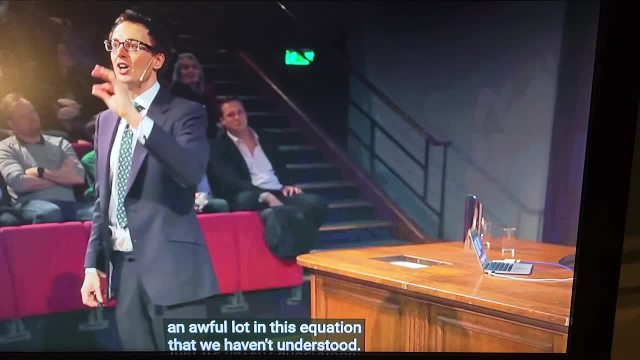 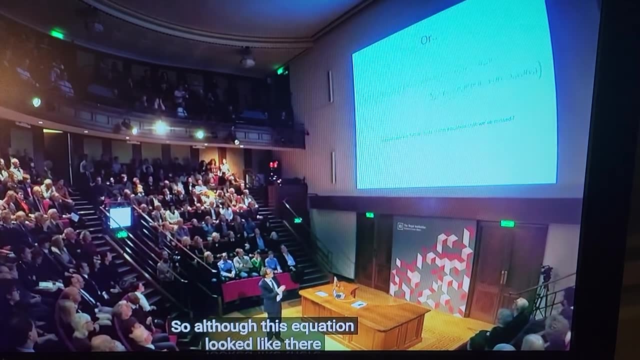 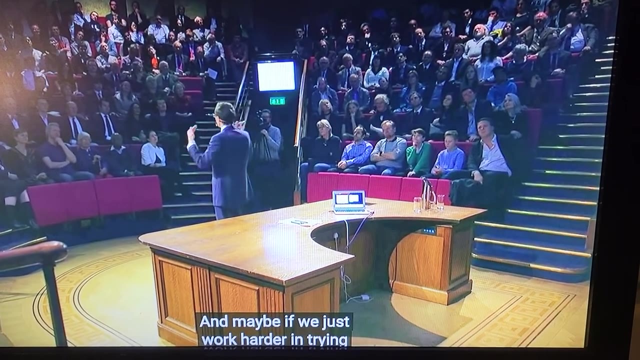 there's an awful lot in this equation that we haven't understood. there's an awful lot to me that's still mysterious in this equation. so, although this equation looked like there were suggestions of unification, maybe they're just red herrings and maybe if we just work harder and 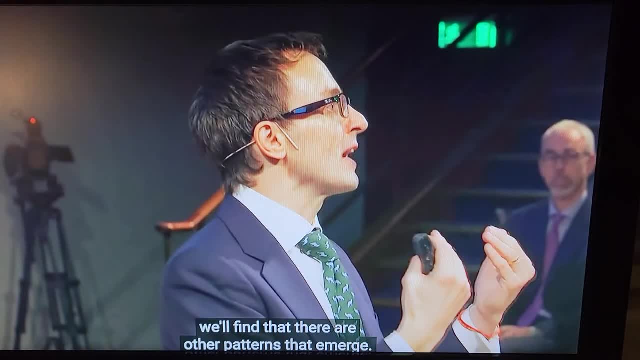 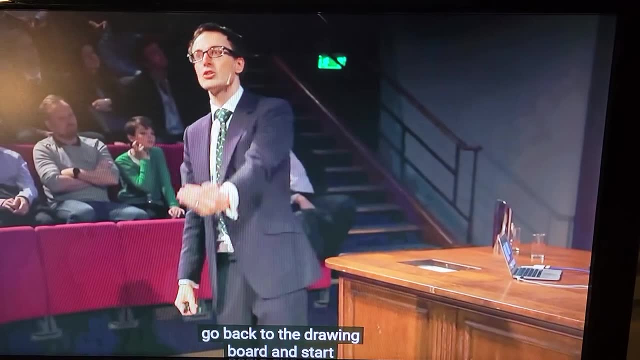 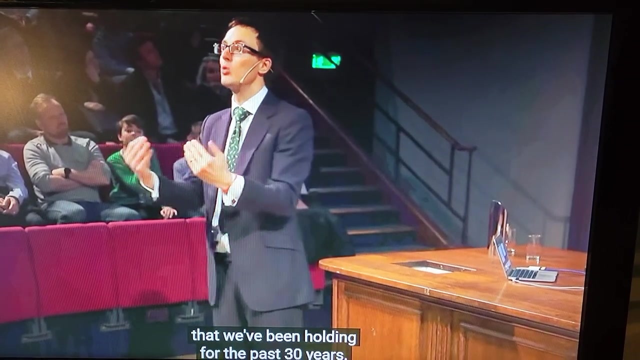 trying to understand this equation more, we'll find that, uh, there are other patterns that emerge. so my response is: i think that maybe we should just go back to the drawing board and, uh, start to challenge some of the assumptions and paradigms that we've been holding for for the